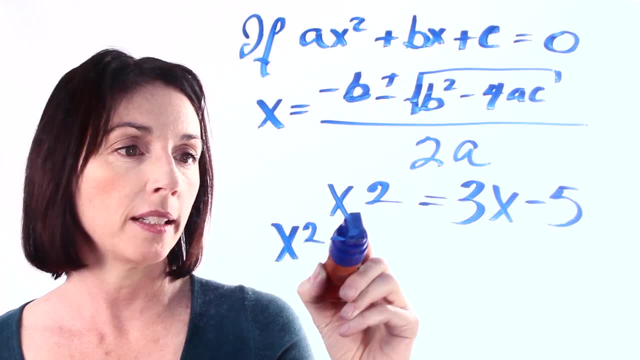 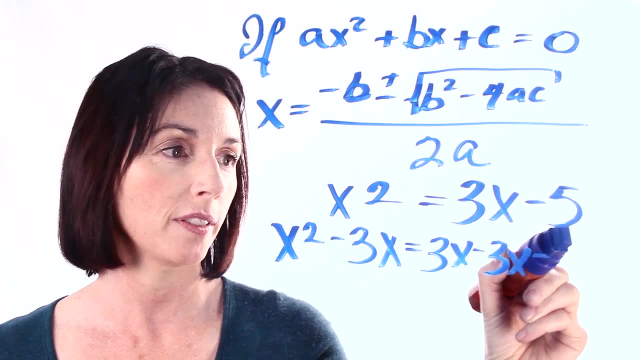 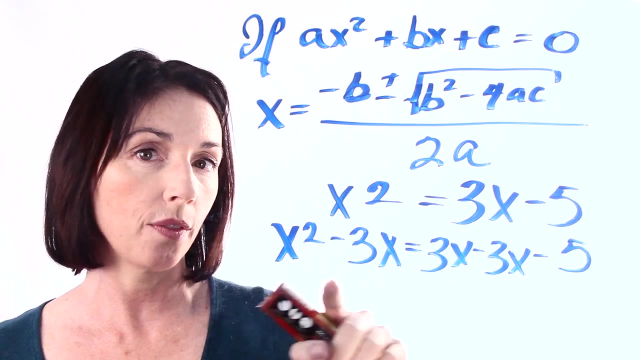 So we have x squared minus 3x equals 3x minus 3x, And we keep our minus 5.. Now 3x minus 3x is just zero, so that goes away. So now what we need to do is we need to get this 5 over to this side. 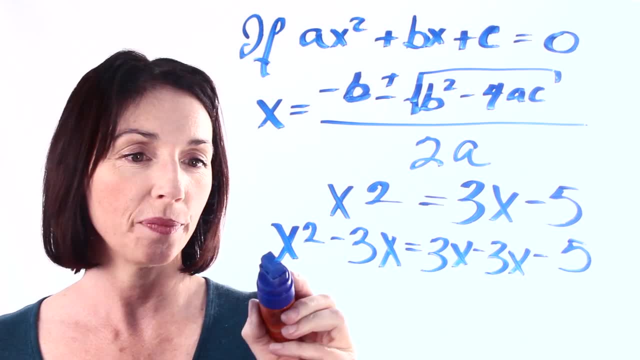 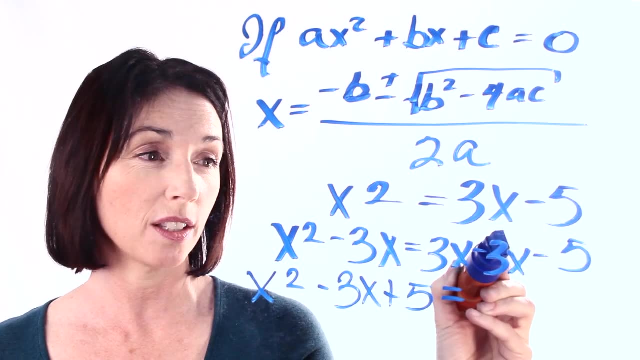 And we can do that by adding 5 to both sides of the equation. So here we go: x squared minus 3x plus 5 equals the 3x, and the 3x just went away- minus 5 plus 5.. 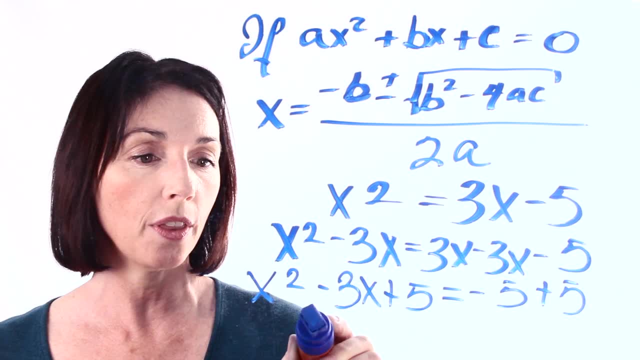 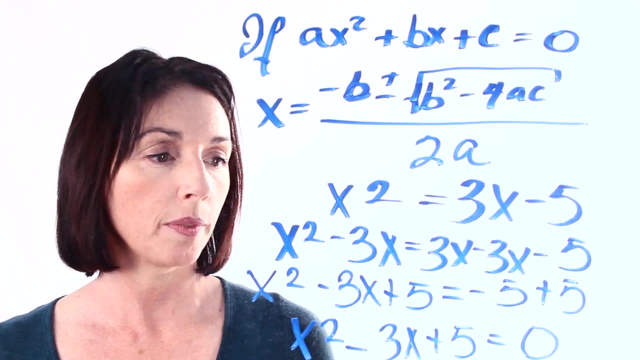 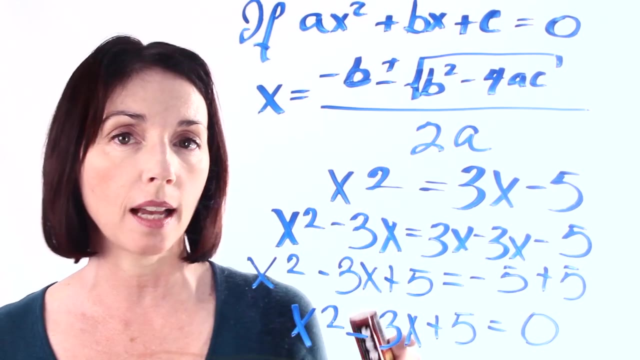 And minus 5 plus 5 is equal to zero. So we end up with x squared minus 3x Plus 5 equals zero. Now we have the right form to satisfy the condition. Now I know we have a minus sign here and a plus sign here, but that's really okay. 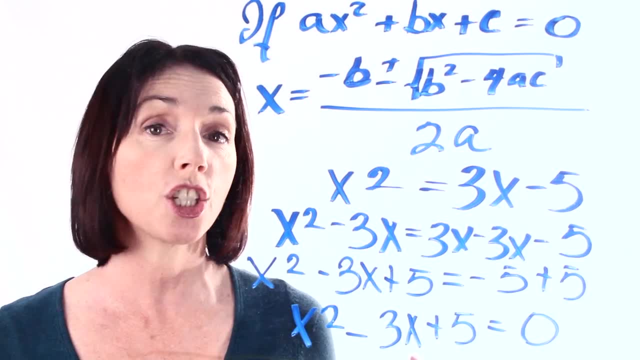 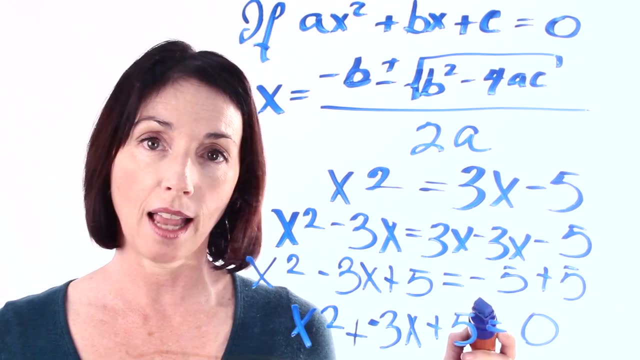 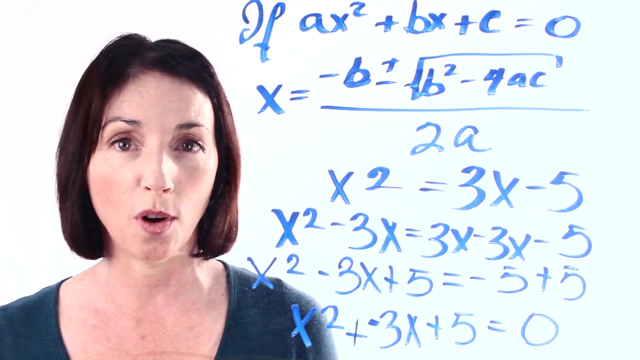 Because we can always change subtraction into addition by just changing the sign of whatever we're subtracting. So minus 3x is the same as plus negative 3x. So our equation is actually in the perfect form to satisfy the condition and we can use the quadratic formula. 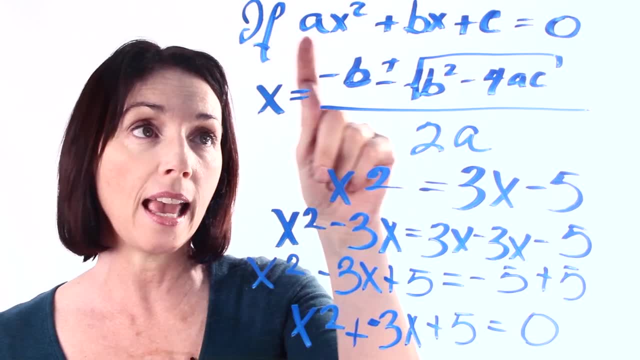 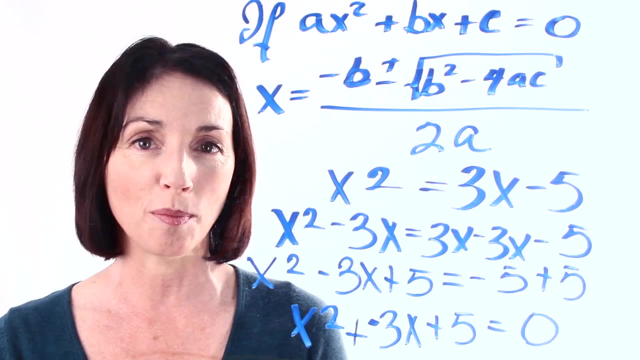 So the next step in the process is identifying a, b and c in the equation we want to solve, and we're going to do that next time, And that's how you satisfy the condition for the quadratic formula. Thanks for learning with me today. 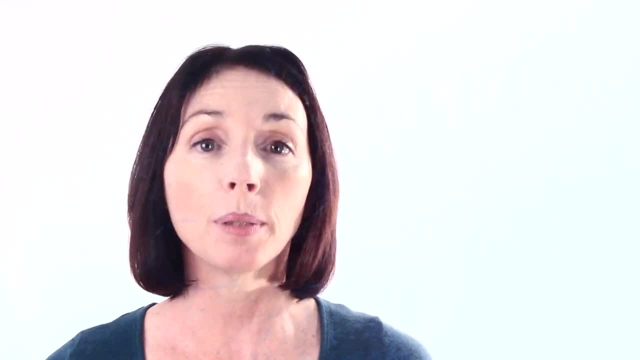 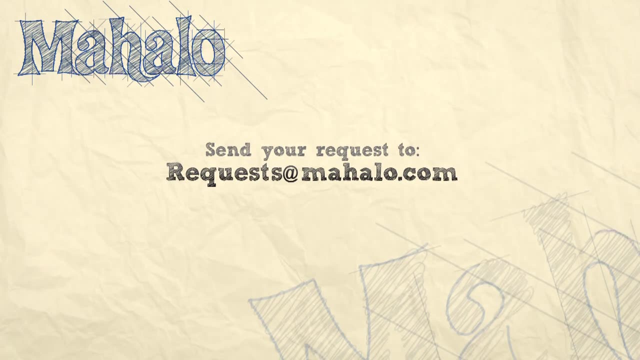 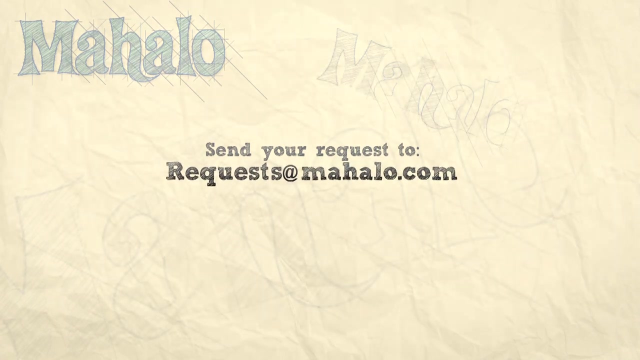 If you have any questions on this topic or anything having to do with math, please click on the links or send us a request to requests at mahalocom. See you later, Thank you.